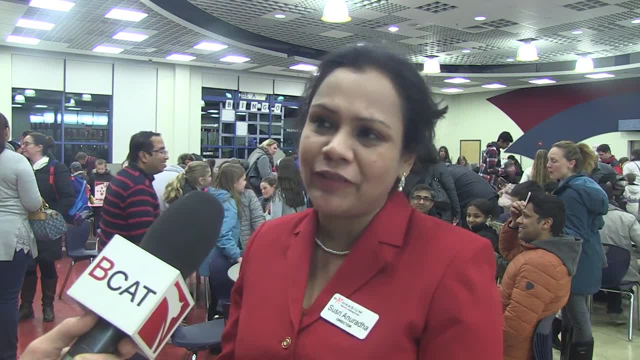 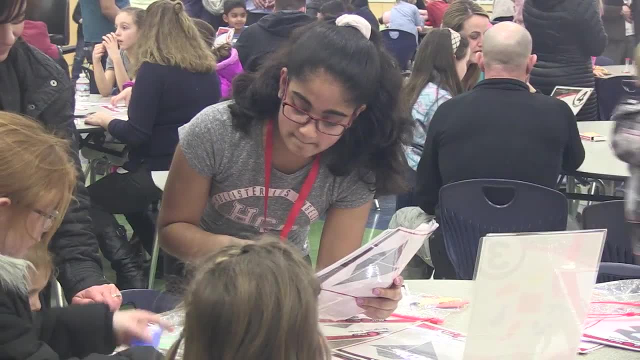 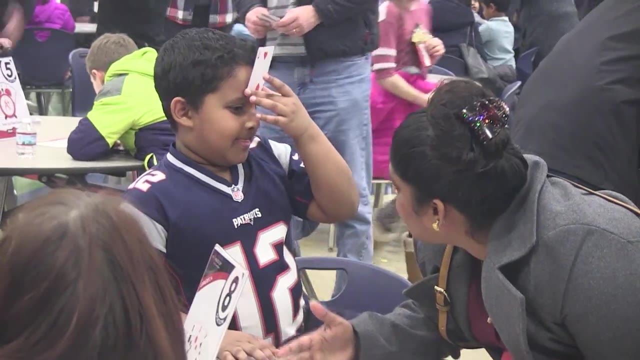 collaborate the kids and the parents together to have a family math night where we can engage the parents as well as the students and play fun math. This is our part of our community outreach effort where we want to show the elementary students how fun math can be, because typically what happens at a 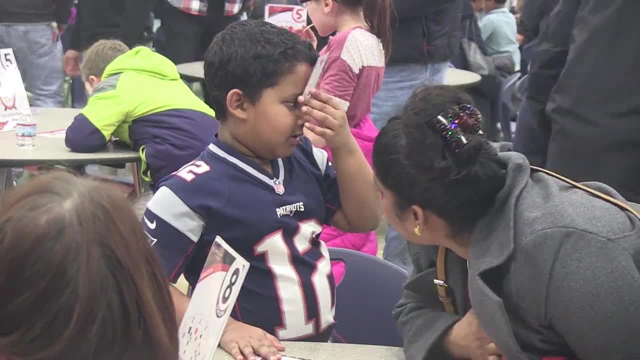 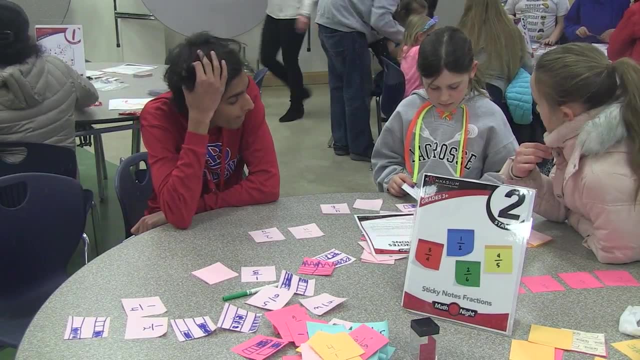 certain age, kids come and say we hate math, we don't like math. So that's why we are doing this kind of effort to show them. math is not just boring worksheets, it's more, can be fun and it has a real-time application where you need. 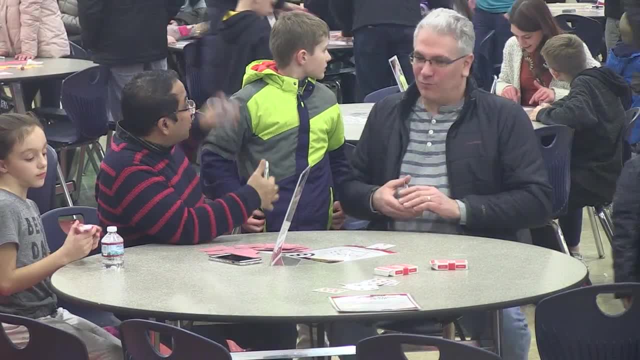 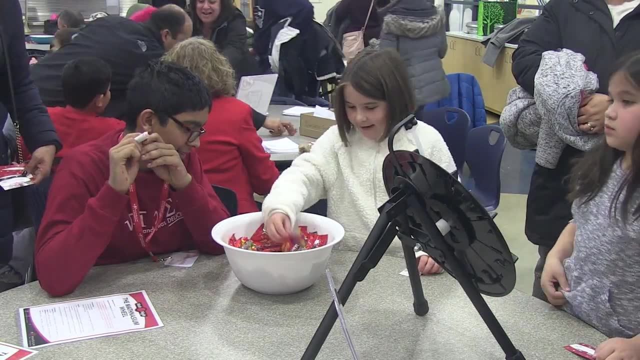 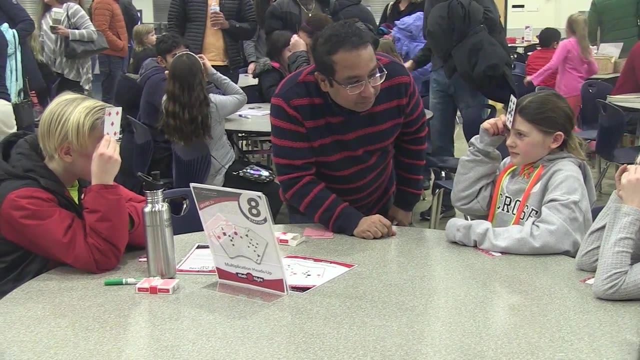 math for your whole life. Before the fun can begin, there are a few preparations Mathanasium has to go through to make it happen. In Burlington we have had four math nights. we have already done two and this is our third one. we have one other one upcoming on February 13th in Francis Wyman. so the 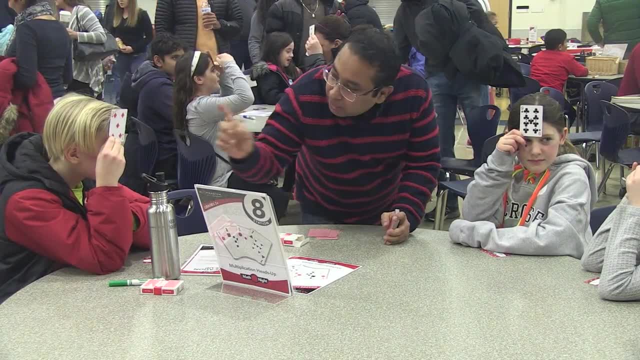 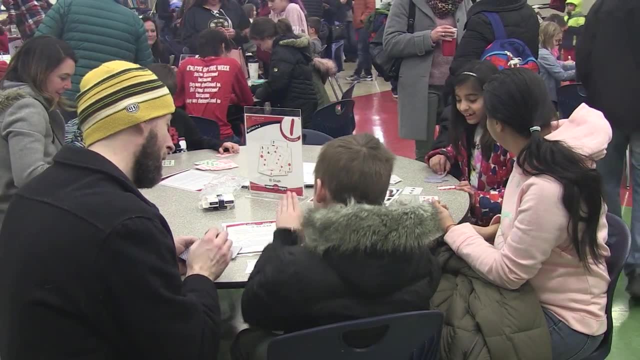 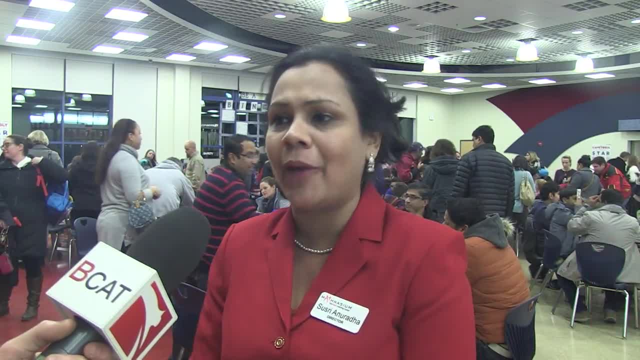 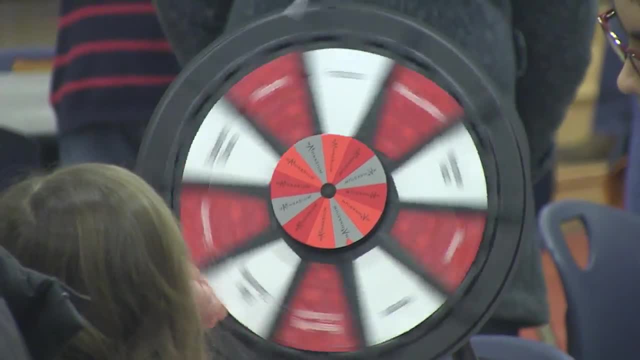 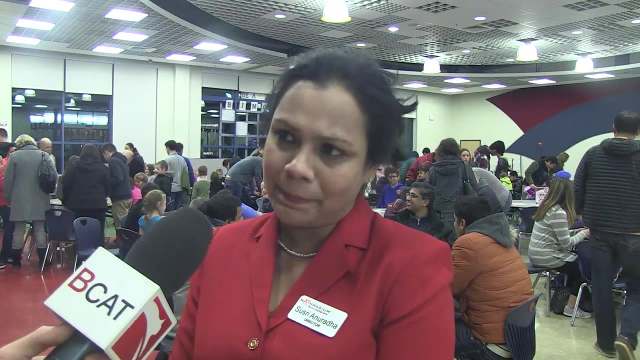 and it's a fun event. it's a free even. come in with your parents and we engage with the students. kids are not the only ones playing the games. parents also get a chance to participate in the academics as well. what we do is that when the parents come in, we give them two things. one is a student passport. what we 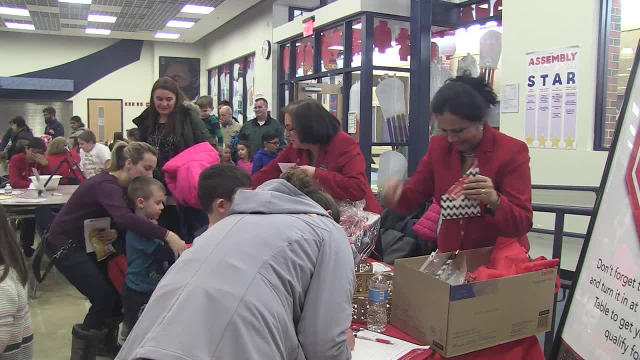 call and another is a parent passport. so parents and students both need to be engaged. so we make sure that they are getting engaged. so we tell the parents. here is your parent passport. you write your name and your name is on the card. so you report back to the students and the students will have your name on the card. 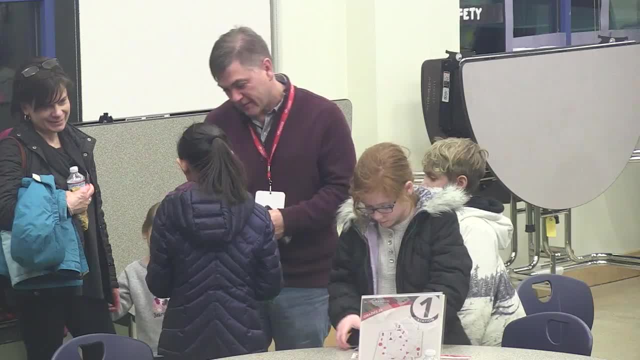 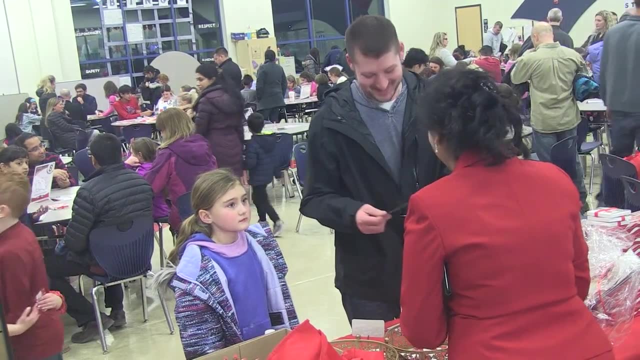 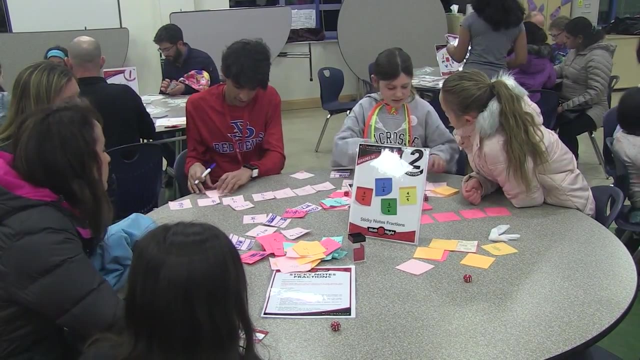 name, you write your details in it and this is your students passport. so you go to the table, you play games with your child there and then you get it stamped. so we have stamps for each table. so when they go and play games, then that table, whoever is the facilitator, they stamp that table thing and they go through ten. 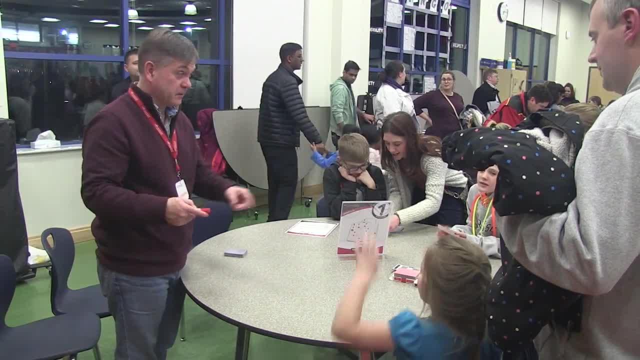 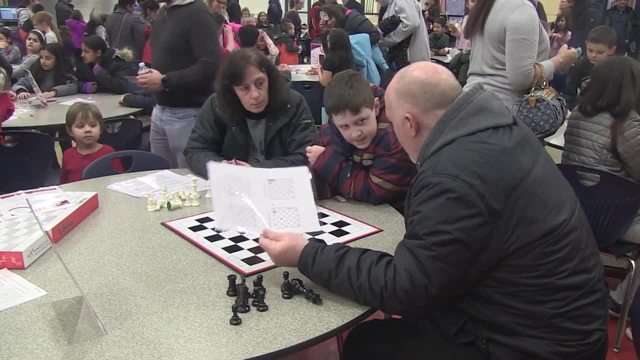 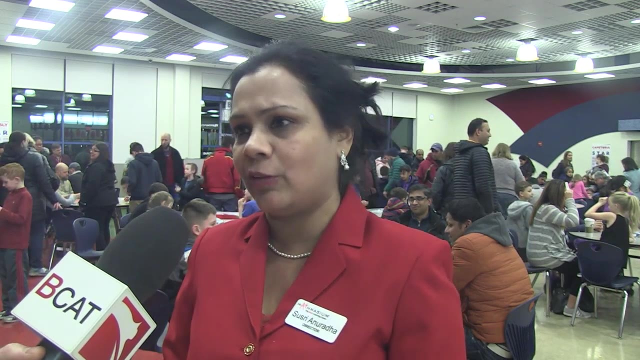 tables. we have around 20 tables here. so based on the grade level, it's kindergarten to grade two is one table and third grade and above is another, because obviously their ability to understand between these two ages are quite different. so we group them as per age appropriate. finally, who said math?